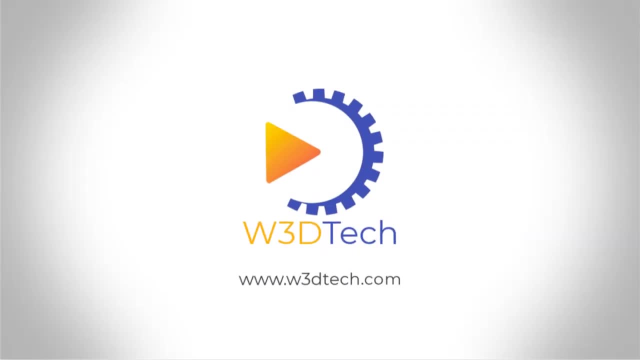 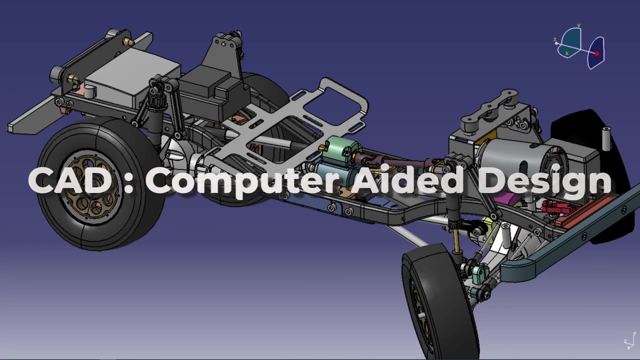 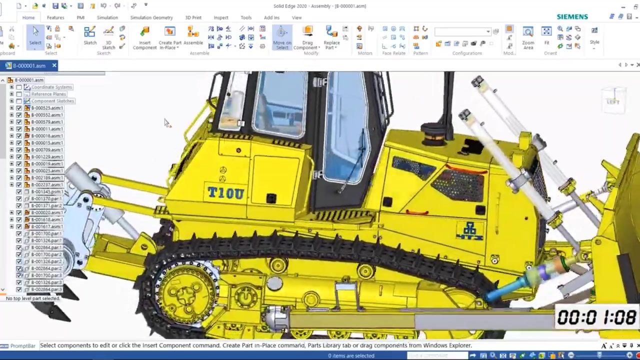 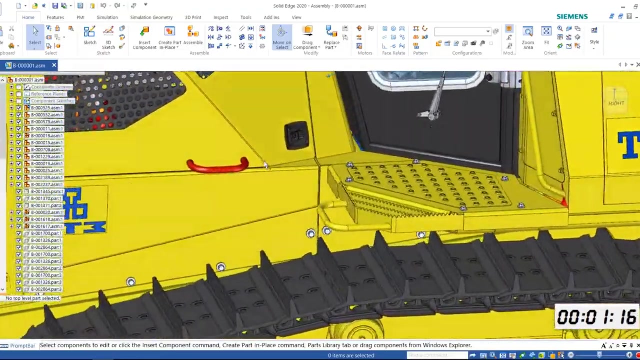 Cade. computer-aided design. Computer-aided design is the process of digitally creating design simulations of real-world goods and products in 2D or 3D, complete with scale, precision and physics properties to optimize and perfect the design, often in a collaborative. 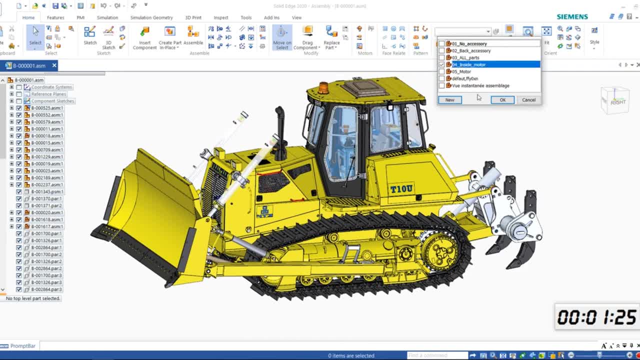 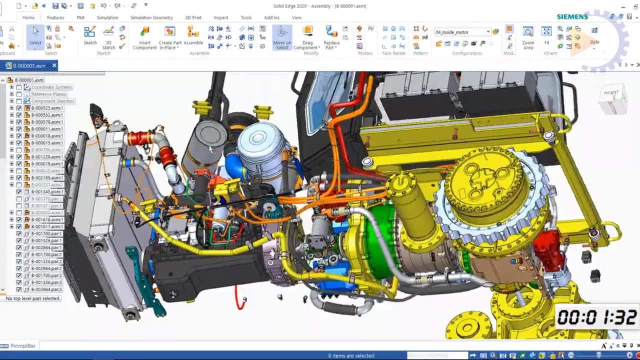 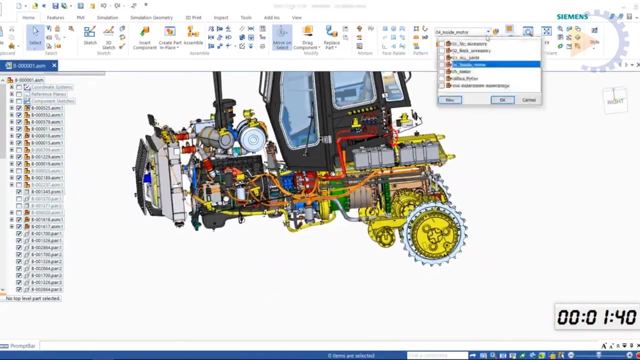 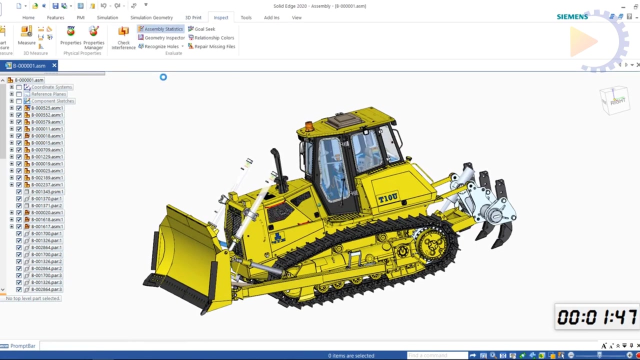 manner before manufacturing. Cade is also sometimes called computer-aided design and drafting. Using computer-based software to assist in design processes is known as computer-aided design. Various kinds of engineers and designers regularly utilize Cade software. Two-dimensional drawings and three-dimensional models can both be produced using Cade software. 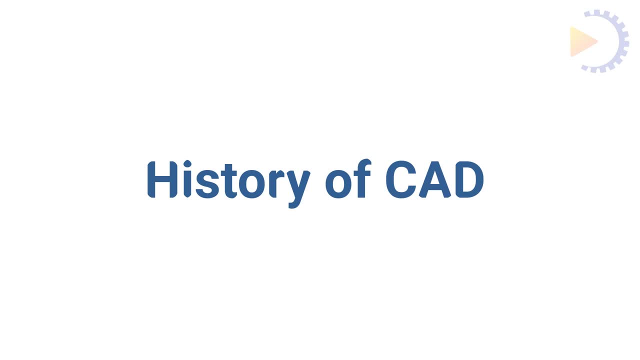 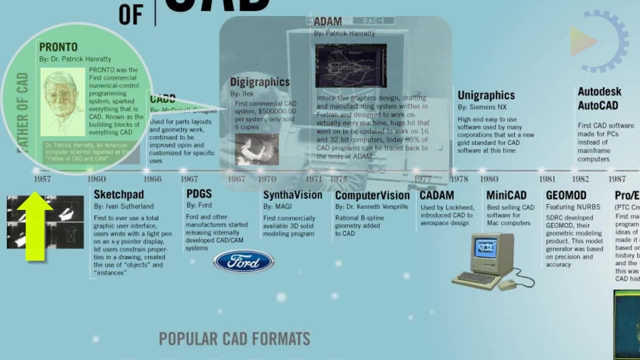 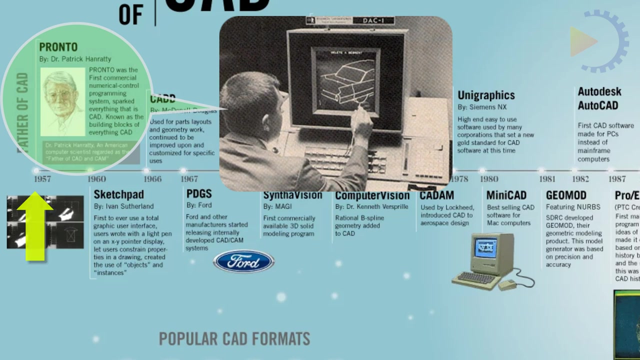 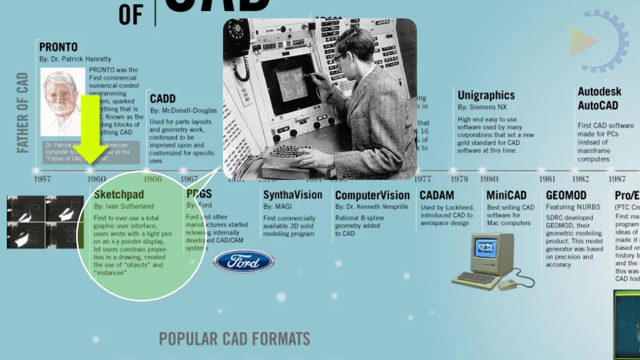 Historical. The first commercial numerical control programming system, Pronto, created by Dr Patrick J Hannity in 1957, is credited with giving rise to computer-aided design. Sketchpad, developed by Ivan Sutherland in 1960 at MIT's Lincoln Laboratory, proved the viability and fundamentals of computer-aided 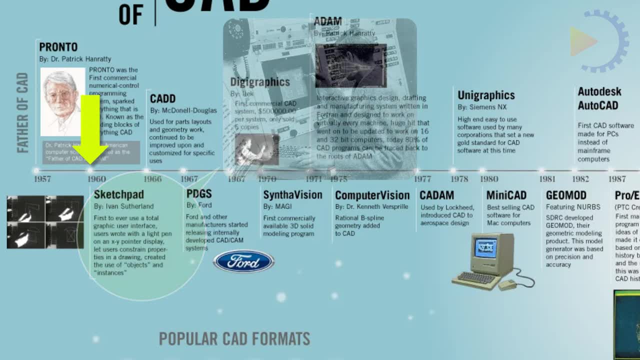 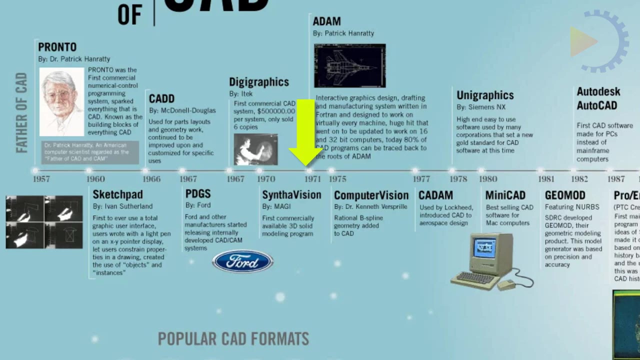 technical sketching Because the machines were so expensive. when Cade was first developed, it was not precisely a viable business option. Engineers may now employ Cade files that accurately depict the object's dimensions and attributes, thanks to the development of many computers and microprocessors in the latter half. 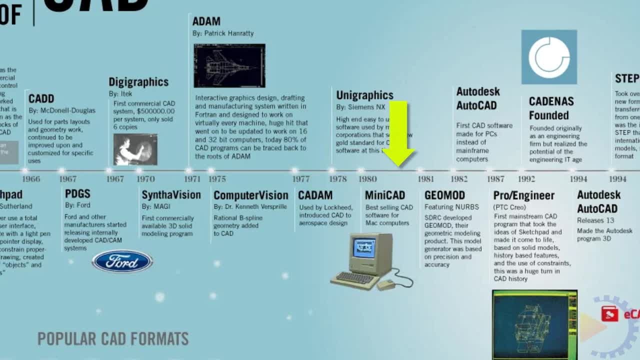 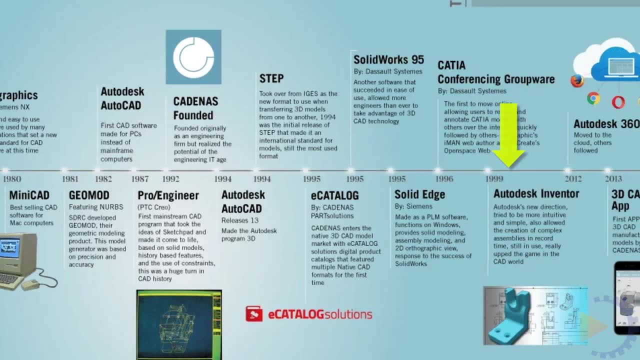 of the 20th century and the resulting increase in computing power, particularly after the rise of cloud computing, We quickly become aware of the importance of Cade in any urban environment made up of objects that all, without exception, were designed before being. 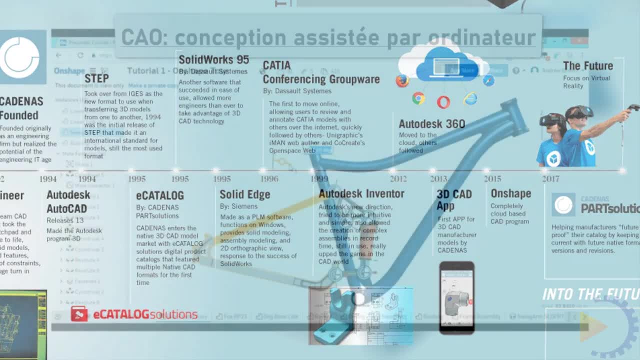 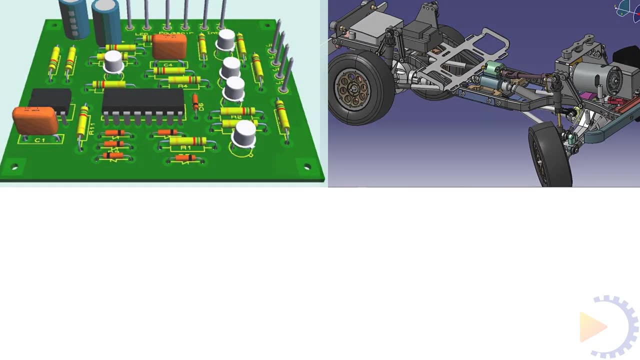 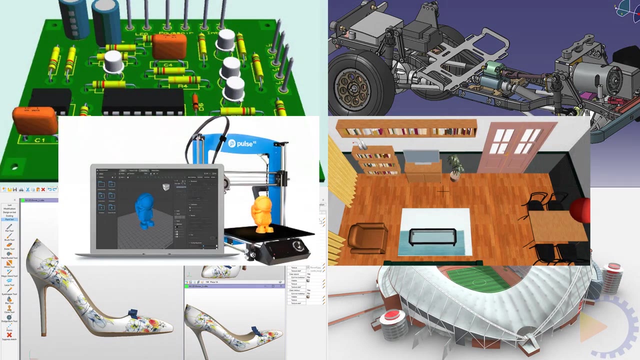 manufactured one day. Who uses Cade? Computer-aided design is used in a wide variety of professions. Cade software is used heavily within various architecture, arts and engineering projects. Cade use cases are specific to industry and job functions. 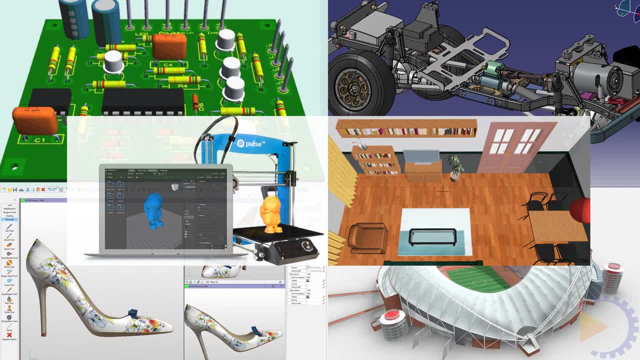 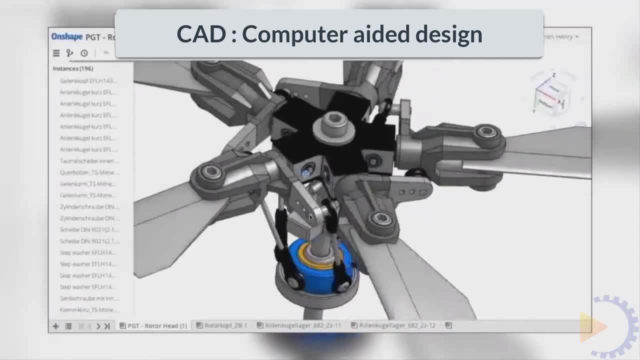 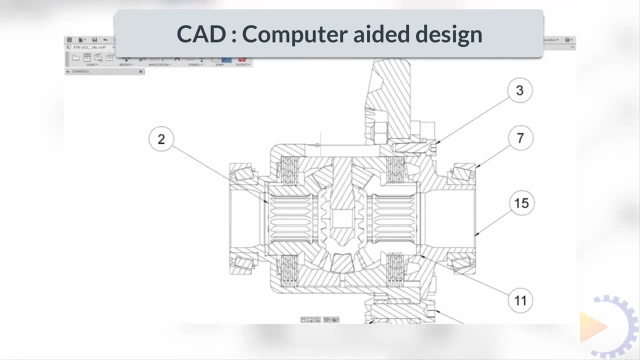 Professions that use Cade tools include, but are not limited to: 1. Mechanical: The field of mechanics is historically one of the first to be equipped, in the 1960s, with Cade software. These allow the designer to express and model a large number of constraints during the design phase of a. 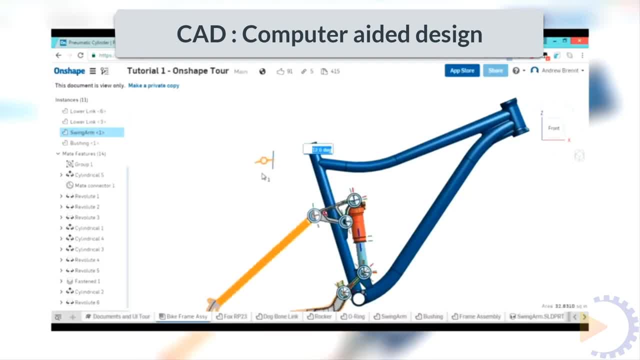 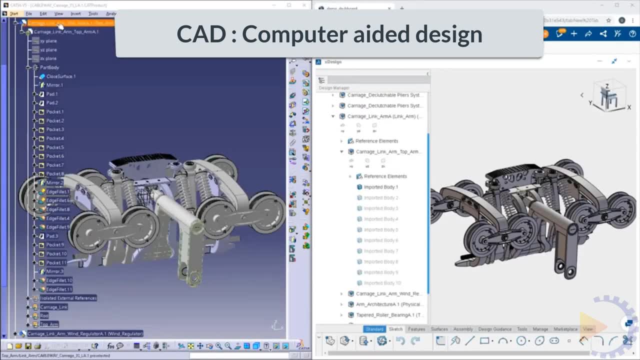 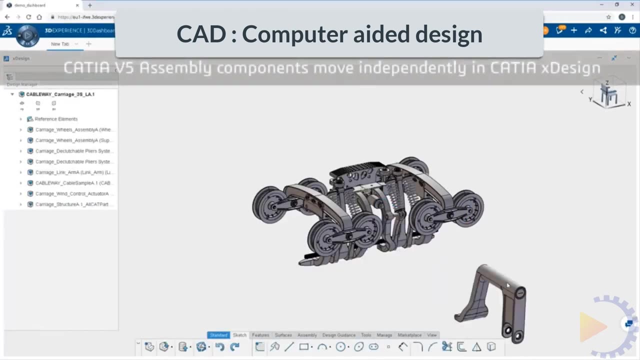 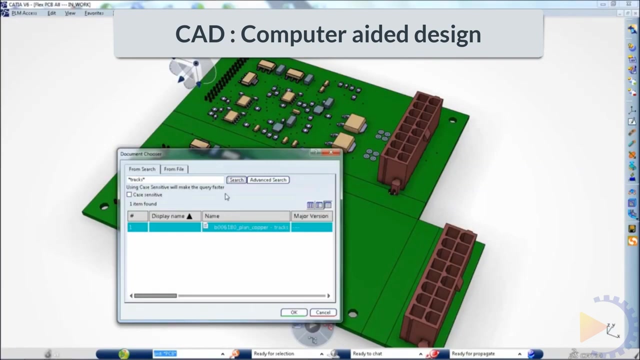 mechanical assembly. The corresponding software is used during one or more development phases, for example product process specifications, sketches, dimensioning, kinematic analyses, dynamic analyses, preparation for manufacturing, etc. 2. Electronics Products also exist for the design of electronic circuits or microprocessors. 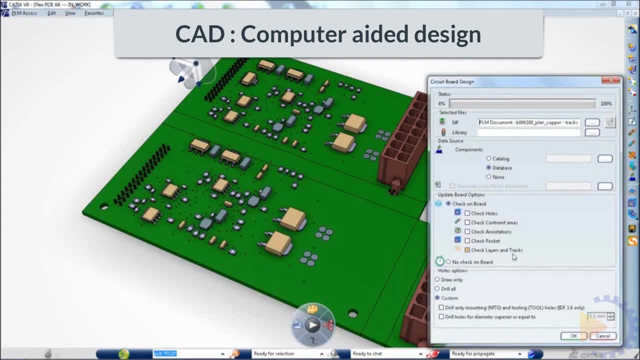 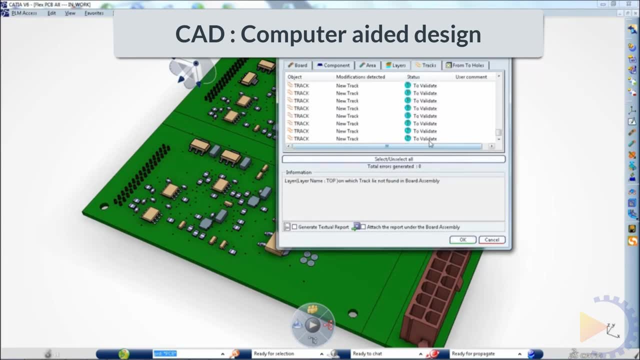 The design of an electronic circuit presents two difficulties. The first, concerning the desired electrical or logical behavior, is certainly the easiest to deal with. We obtain a computer model of the diagram, built as on a Cade tool. However, each component is affected by a law of behavior which provides a virtual model allowing 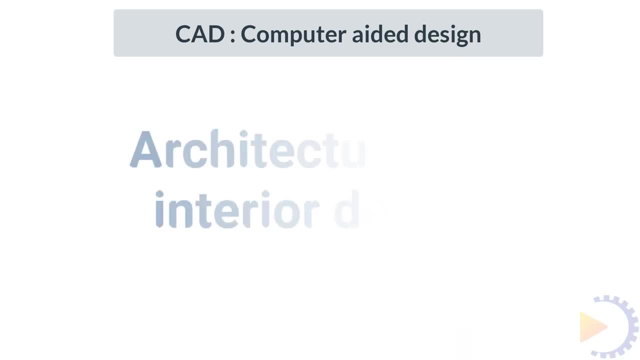 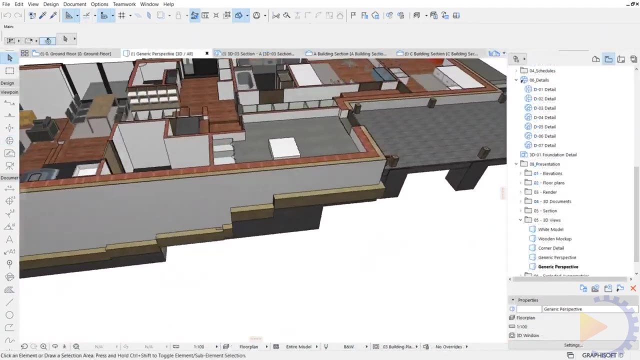 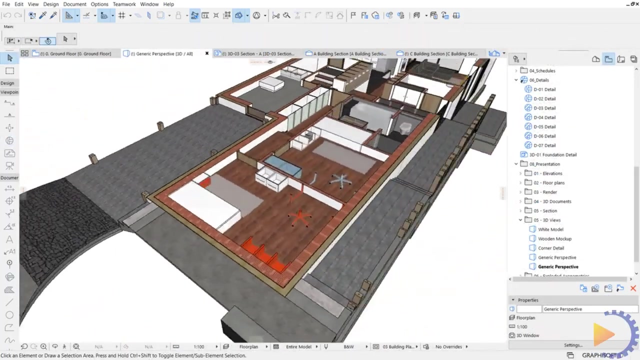 operation tests. 3. Architecture and interior design. Animations and other presentational materials can also be produced using Cade, which can also be used to construct 2D or 3D representations. Detailed instructions on how to make something are delivered through technical drawings. 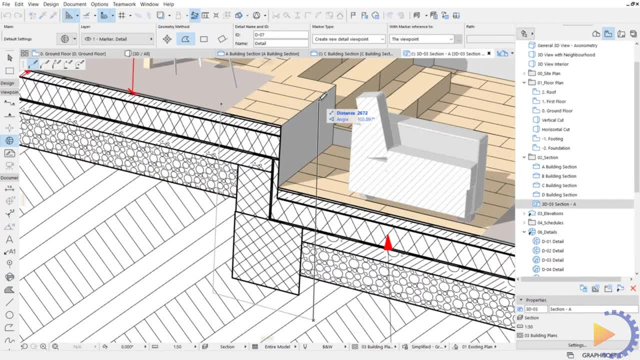 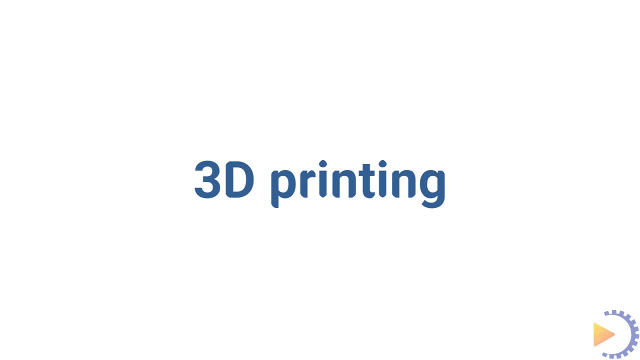 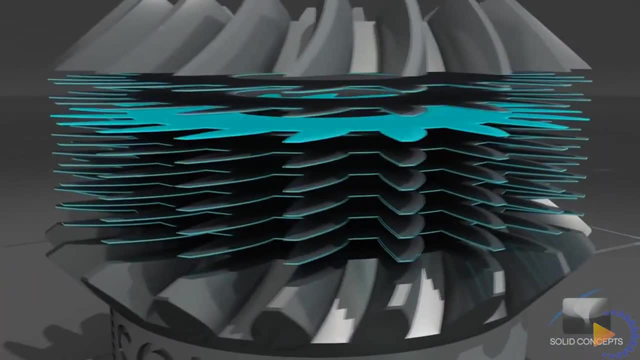 Designs for mechanical engineering and architectural structures can be included in technical drawings using Cade. 4. 3D printing: Creating a three-dimensional real-world object from a digital model can be done via a process called three-dimensional printing. It is accomplished by using an additive technique that involves drawing a 3D model. 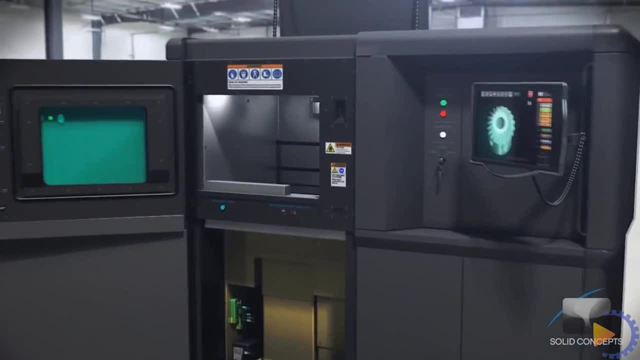 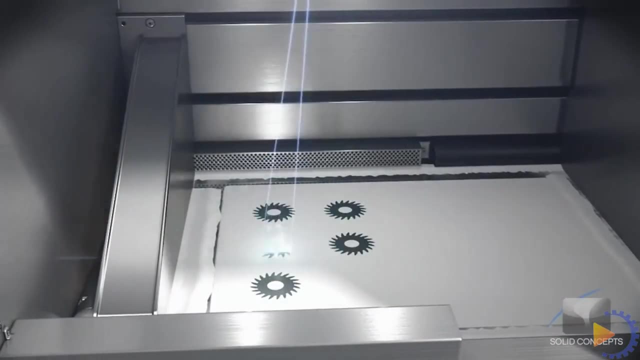 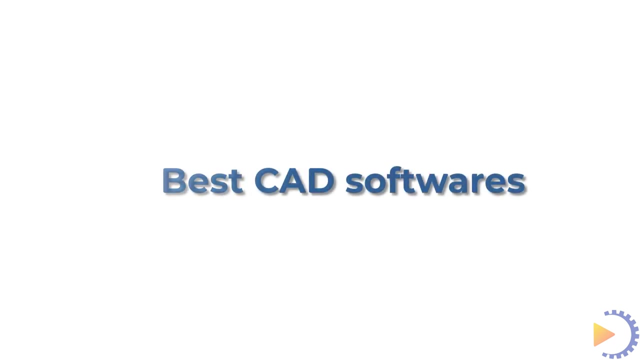 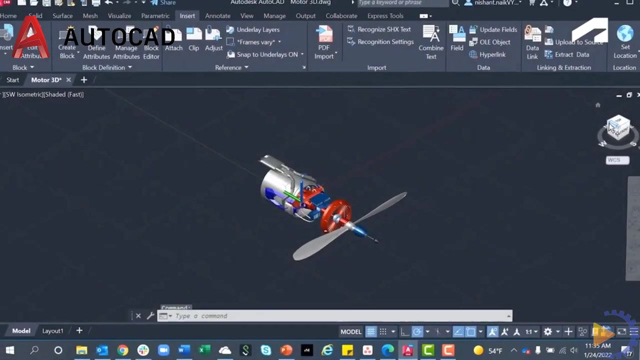 It is a technique that involves building up layers of material, typically thermoplastic, and succession. A horizontal cross-section of the ultimate object is represented by each layer, which is finely sliced. Examples of Cade software: AutoCade. one of the first Cade software to hit the market was AutoCade from Autodesk, which has a strong reputation in several industries. 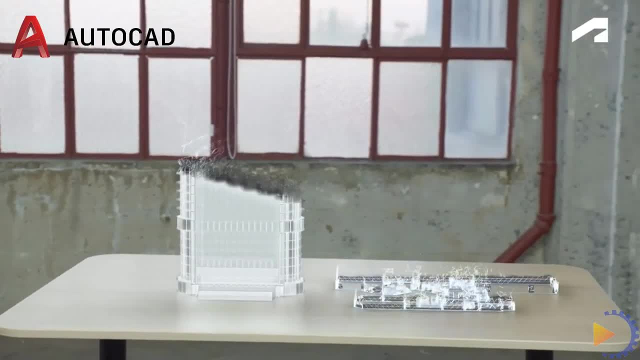 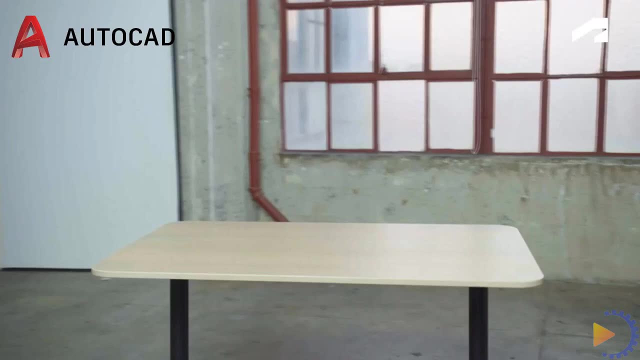 This Cade program is a product of a company called AutoCade, Cade's Artsive Automники. Cade program is a product of an automatic softwareechoing company based in Lahore, in Transnistria. Automatique of the technology is a product of an interesting industry. 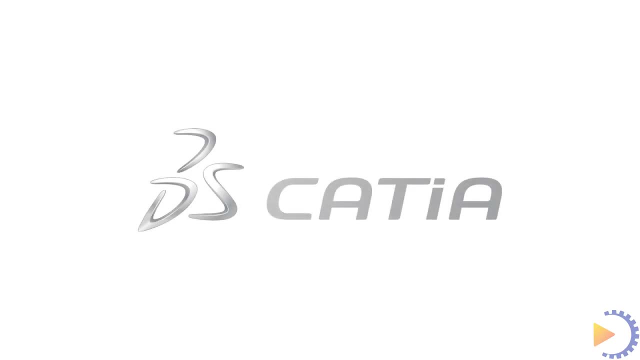 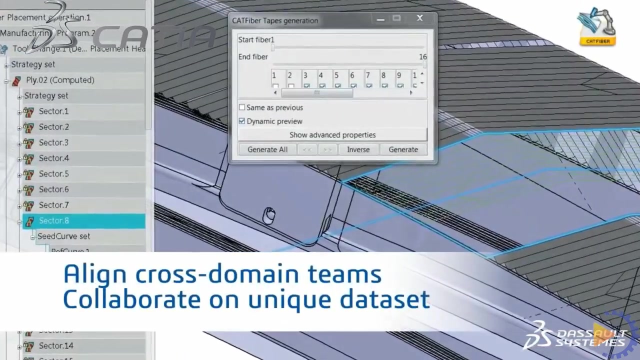 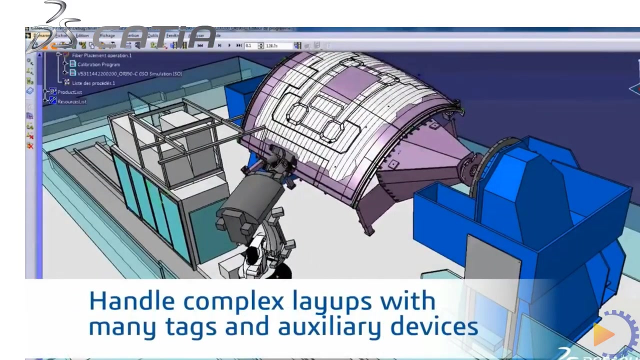 Why should driving ludicrous cars, cats problems andcompl bar importantes to the disbeliving client? It involvesstationihanat Faculty of Aquaculture University or International hierarchy Sigma. My name is Kevin Mther Zilker. I am a professor of Sociology at MIT, Toronto. 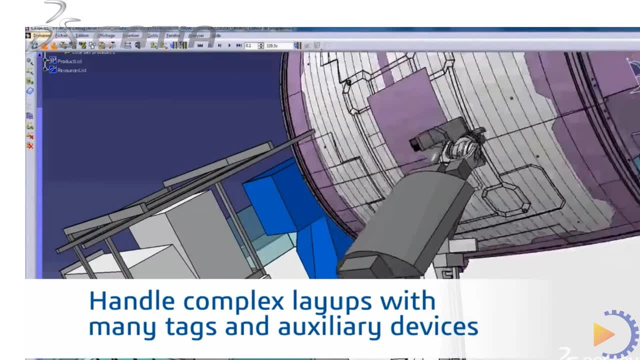 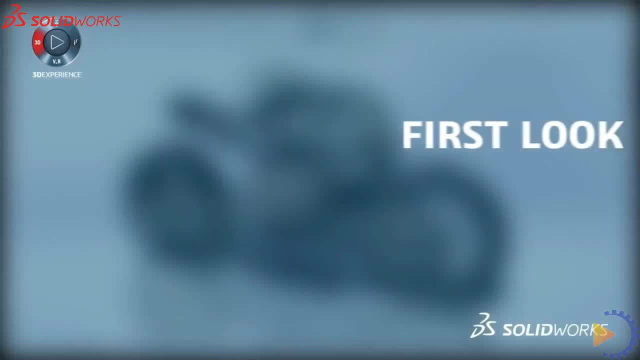 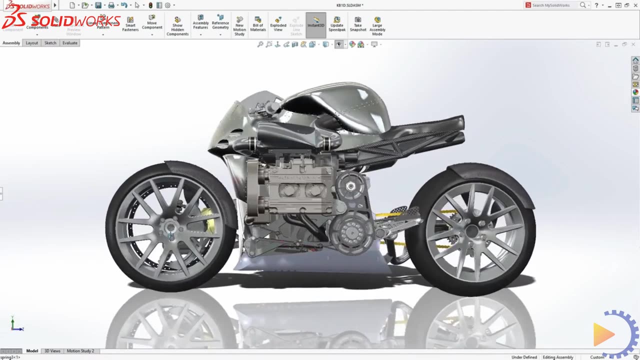 My research field is mechanical engineering by the French company Dassault Systèmes SOLIDWORKS. professional 3D designers frequently utilize this Dassault Systèmes product. It is a feature-based parametric model. Employers usually look for candidates with SOLIDWORKS knowledge. 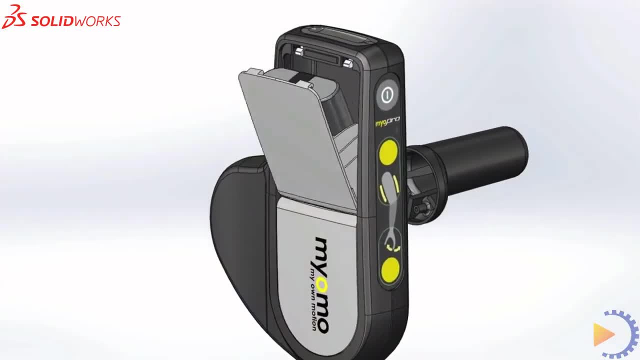 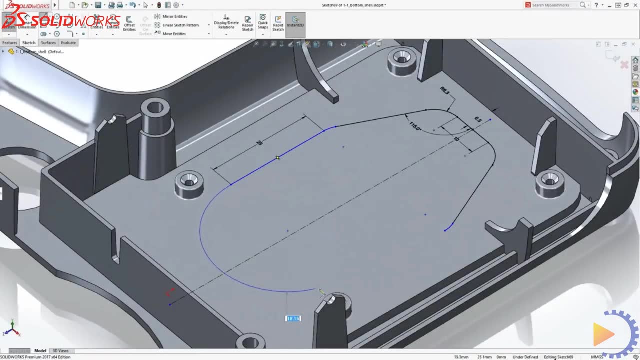 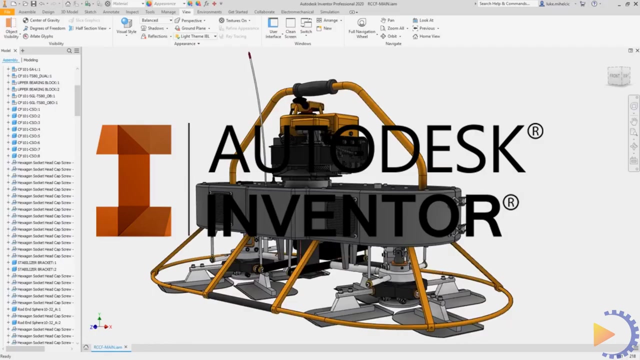 because it is a well-known mechanical design software with a sizable user base. This 3D modeling CADE software is widely utilized in the mechanical engineering and design fields. Inventor, the Autodesk-provided CADE software, is a powerful program built specifically for mechanical design. 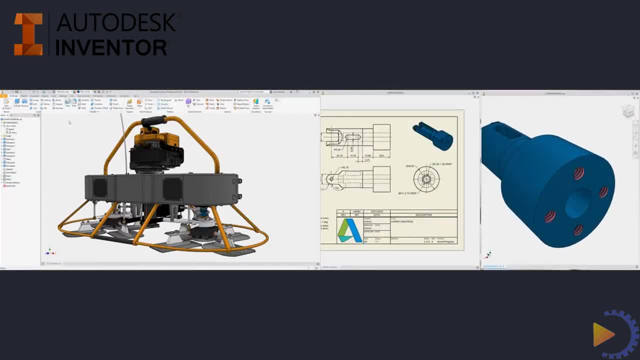 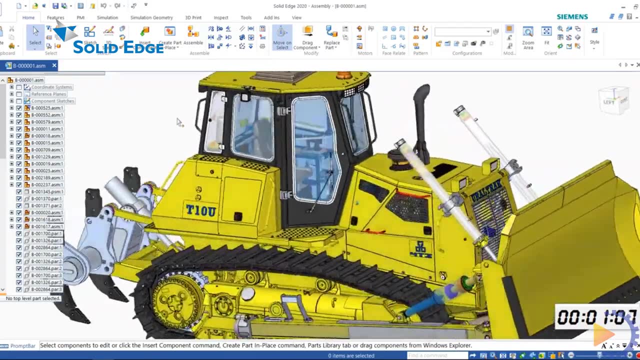 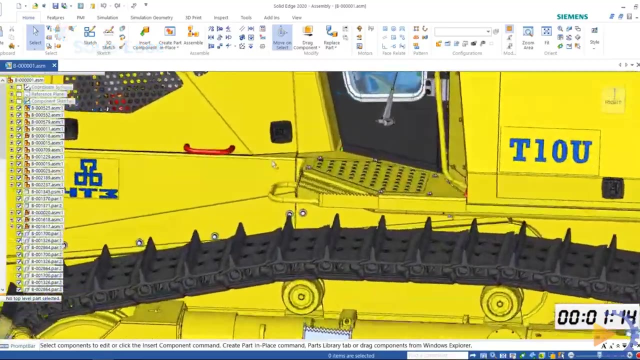 making it a specialized tool for 3D design documentation and product simulation. SOLIDEDGE, developed by Siemens as a PLM software, functions on Windows, provides solid modeling, assembly modeling and 2D ordering. This is a high-quality orthographic view. 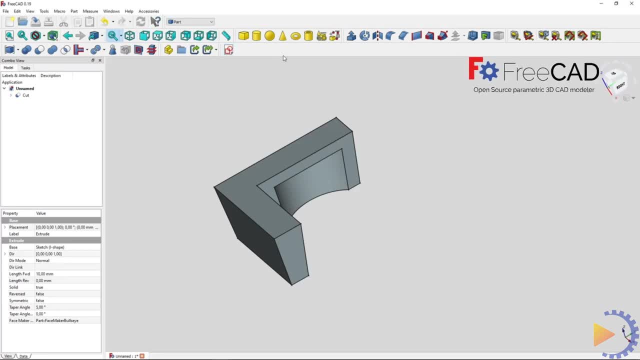 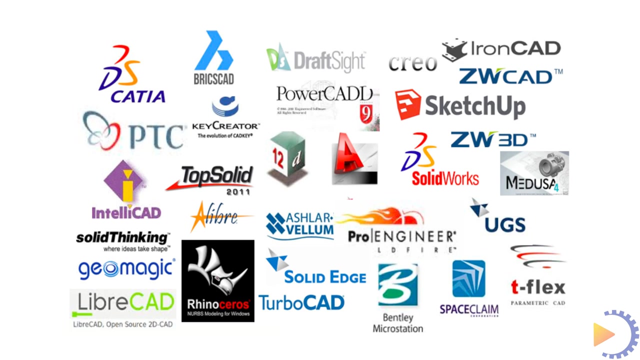 FreeCADE. FreeCADE is an open-source parametric modeler that excels in all vital CADE applications, including product design, mechanical engineering and architecture. Share with us your favorite CADE software. Thank you for watching this video. Don't forget to subscribe.